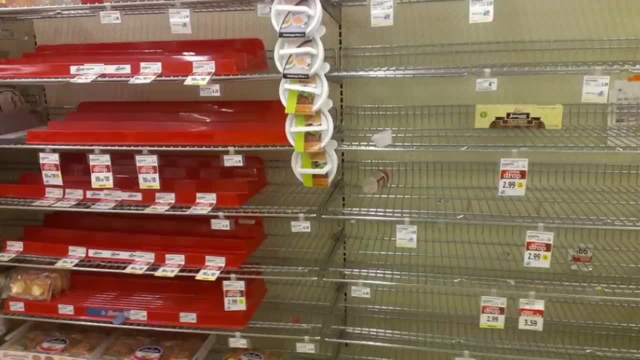 pretty crazy, huh. There's a lot of empty space on these shelves. This is called a shortage. A shortage is when there is not enough for sale. at the current price There's not enough items to sell, So when somebody comes by and wants to buy one of these items, they can't. 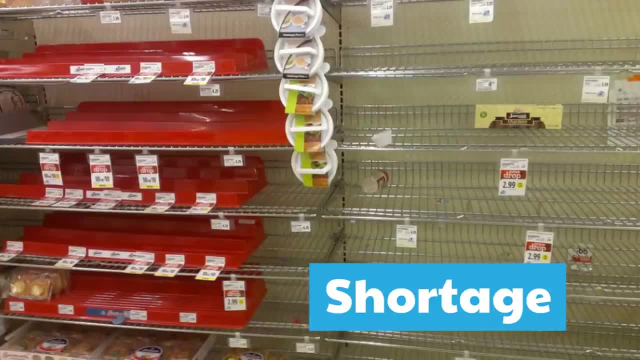 because they're not going to be able to buy it. So when somebody comes by and wants to buy one of these items, they can't because they're not going to be able to buy it. So there's not enough for sale at the current price. These are bananas, A lot of bananas. 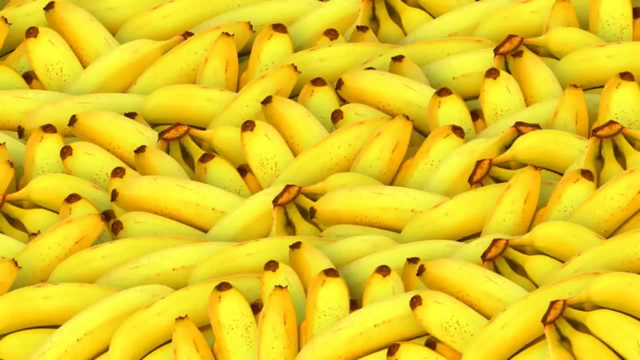 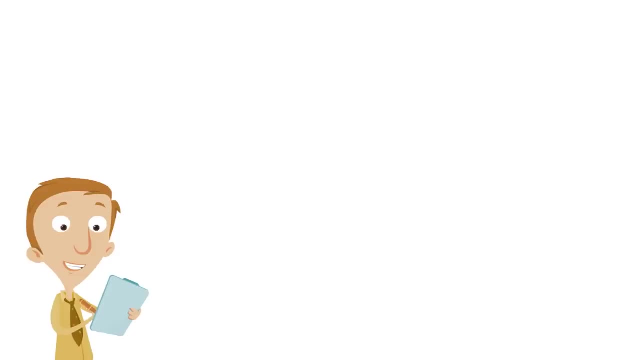 Tons and tons of bananas. In fact, this might be too many bananas for the store to sell. This is called a surplus. That's when there is too much for sale at the current price. You see, a shortage is when there is not enough for sale at the current price. 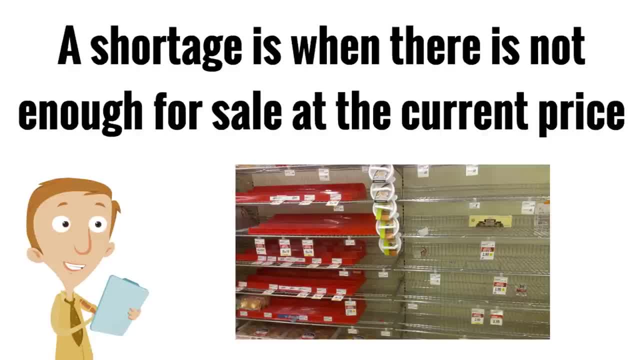 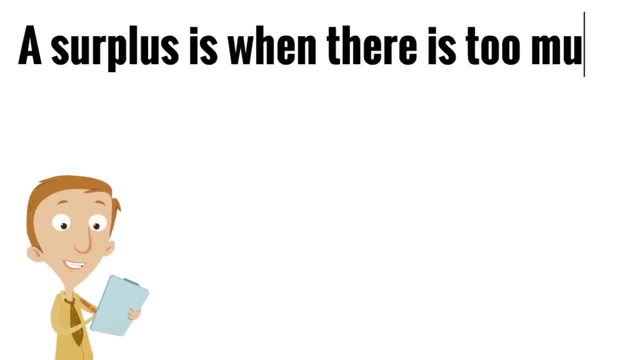 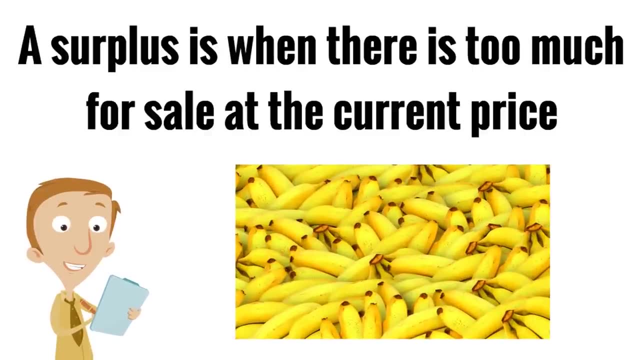 Like these empty shelves. This is a shortage, But a surplus is the exact opposite. A surplus is when there is too much for sale at the current price. Our example are the bananas. These bananas are all ripe and they're ready to turn. They need to get sold, and sold quickly, to different families and people that want to eat. 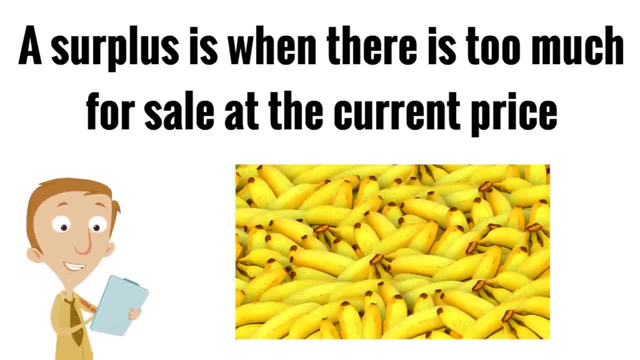 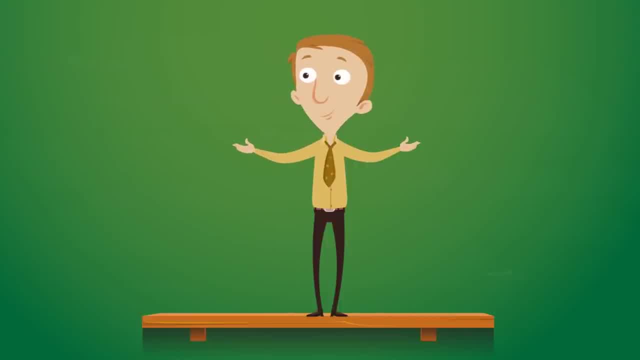 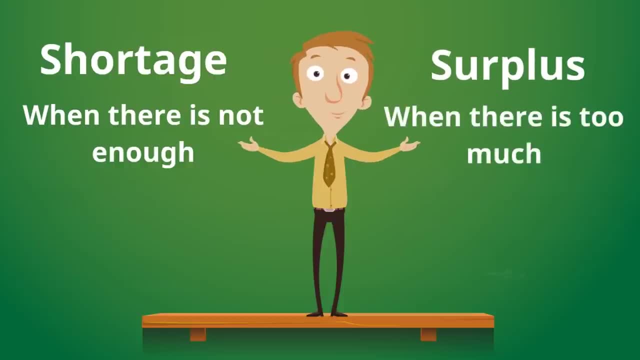 bananas. But a surplus is when you have too much for sale. There are too many bananas. Another way of putting it: a shortage is when there's not enough. A surplus is when there is too much. So stores and people who sell goods and services want to make sure that they're right in. 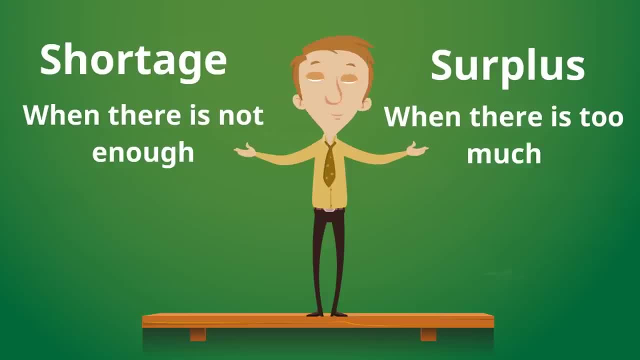 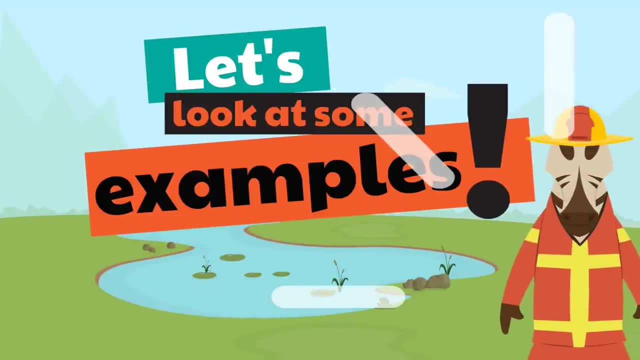 the middle. They don't want to have a shortage, but they don't want to have a surplus either. They want to be right down the middle, because a shortage there's not enough And a surplus there's too much. Hey, let's look at some examples. 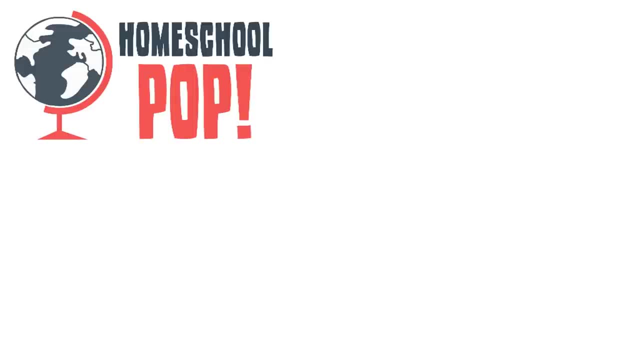 We're going to look at some situations and decide: is this a shortage or a surplus, Shortage or surplus, And you can help us out. Are you ready? Cool, Let's get started. Let's say a store has six computers that they want to sell. 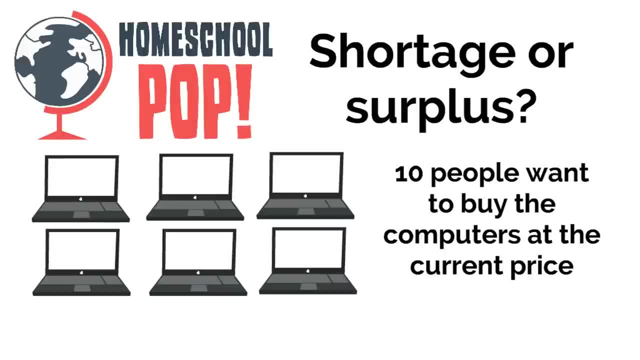 And there are ten people who want to buy the computers at the current price. So six computers and ten people who are willing to buy it at the current price. Is there a shortage or surplus? Is there a shortage or surplus? Yeah, a shortage. 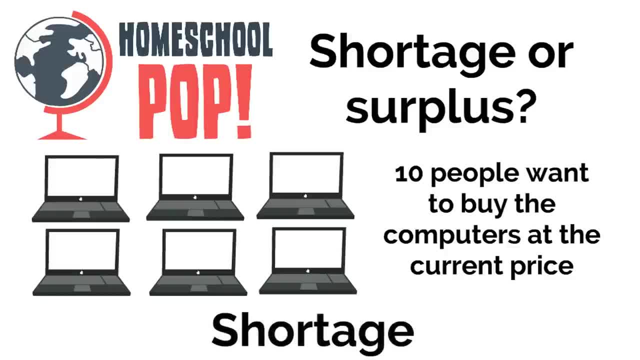 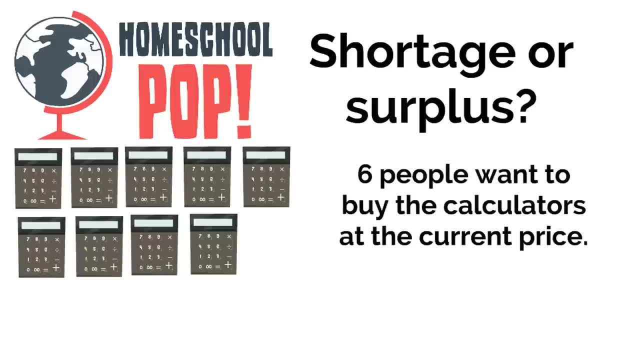 There are not enough computers to sell to everyone who's willing to buy them at the current price. They need to make sure they have more computers to sell so there's no longer a shortage. Let's try this one. Let's say an office store has nine calculators that they are selling. 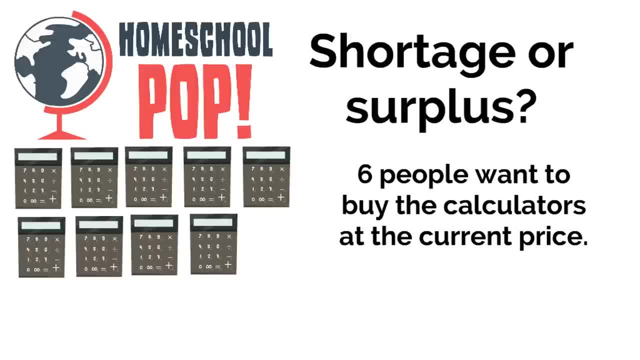 And let's say there are six people who want to buy the calculators at the current price. So there are nine calculators and there are six people who are willing to buy the calculators at the current price. Is there a shortage or surplus? 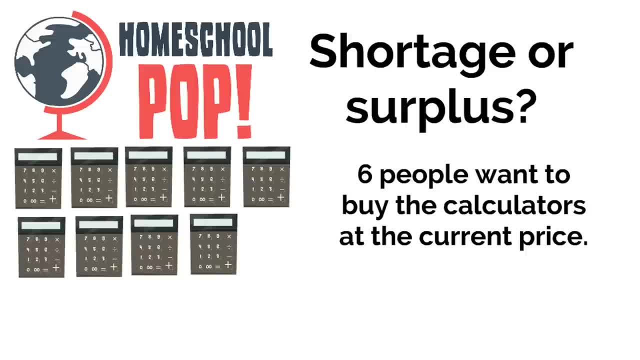 Is there a shortage or surplus? Uh-huh, a surplus. There are too many calculators to sell. The store might need to lower the price of the calculators, so more people are willing to buy the calculators and there would no longer be a surplus. 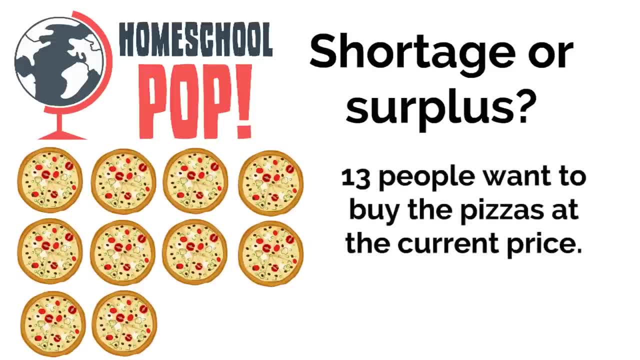 Ah, a pizza shop. Let's say a pizza shop has ten pizzas and there are thirteen people who want to buy the pizzas at the current price. So there are ten pizzas and there are thirteen people who want to buy the pizzas. So there are ten people who want to buy a pizza at the current price. 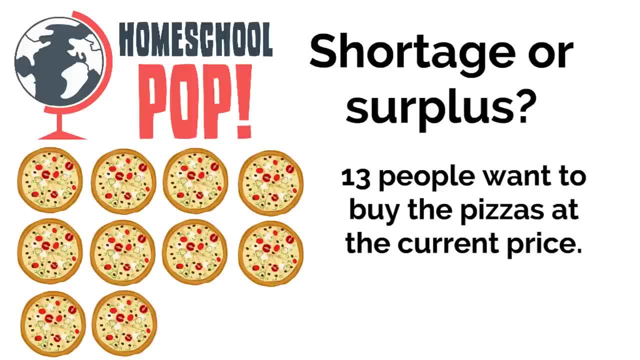 Is there a shortage or surplus? Is there a shortage or surplus? Yeah, a shortage. There are not enough pizzas to sell to everyone who's willing to buy at that current price. They need to make more pizza. so there's no longer a shortage. 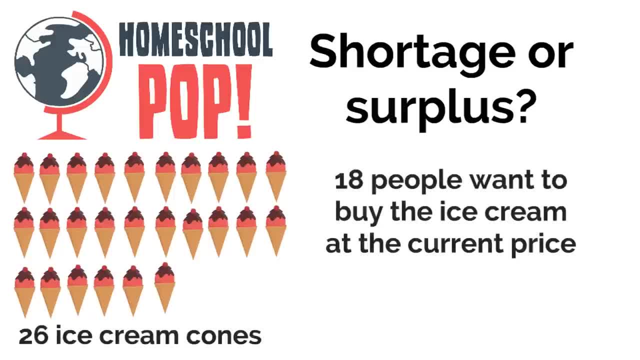 Our last example is an ice cream shop, Mmm tasty. Let's say there are twenty-six ice cream cones available for sale and there are eighteen people who want to buy the ice cream at the current price. Interesting situation: Twenty-six ice cream cones, eighteen people who are interested in them. 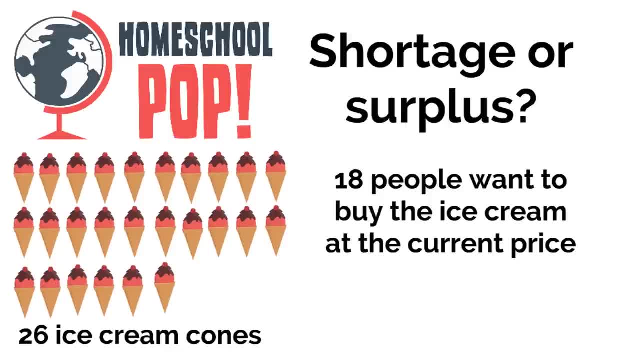 Is there a shortage of ice cream cones or a surplus of ice cream cones? Hm, Which is it, Shortage or a surplus? Is there a shortage of ice cream cones or a surplus of ice cream cones? OK, OK, Ya. 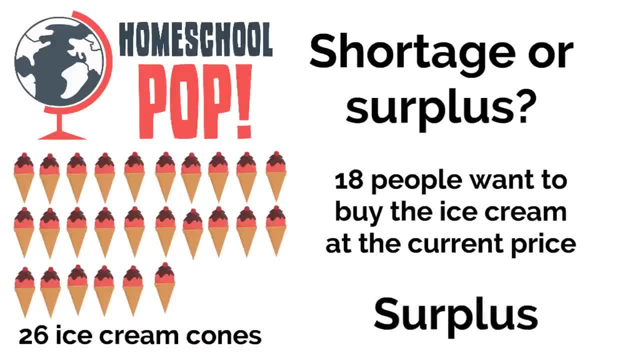 A surpluss. There are too many ice cream cones to sell And the ice cream shop might need to lower their prices So that more people are willing to buy ice cream cones. and there won't be a surplus, because guess what? The ice cream is gonna melt. 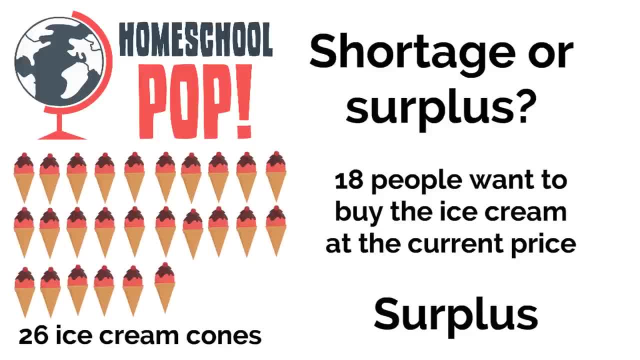 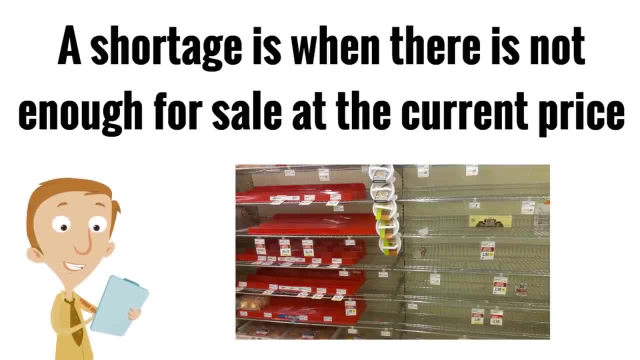 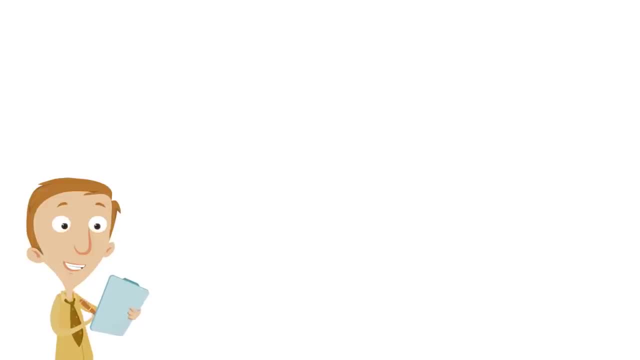 The ice cream is gonna melt. To review: a shortage is when there is not enough for sale at the current price, just like this picture of the empty store shelves. this is a shortage. a surplus, however, is when there is too much for sale at the current price. our example were the: 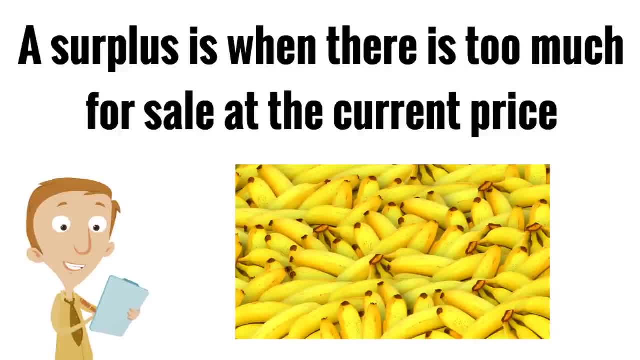 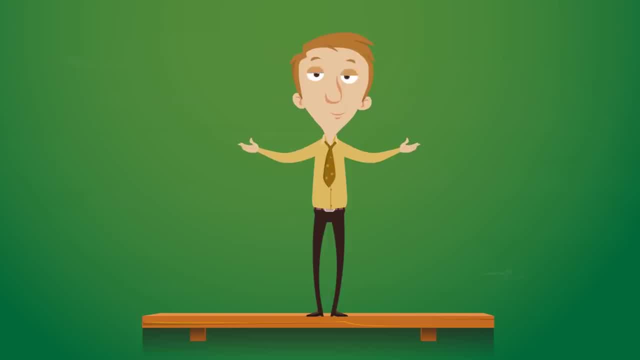 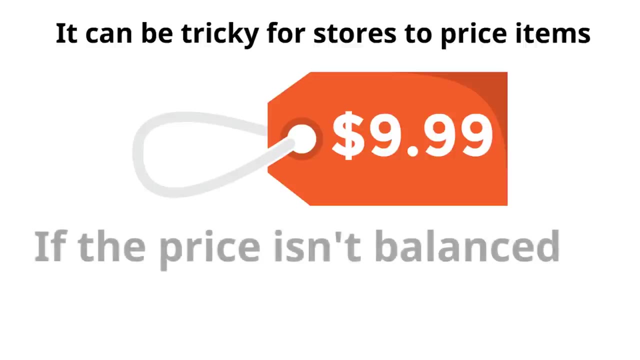 bananas that need to get sold and it looks like there might be way too many. that is a surplus. an easy way of looking at it is: a shortage is when there is not enough. a surplus is when there is too much. you know it can be tricky for stores to price items. if the price isn't balanced, there can be a. 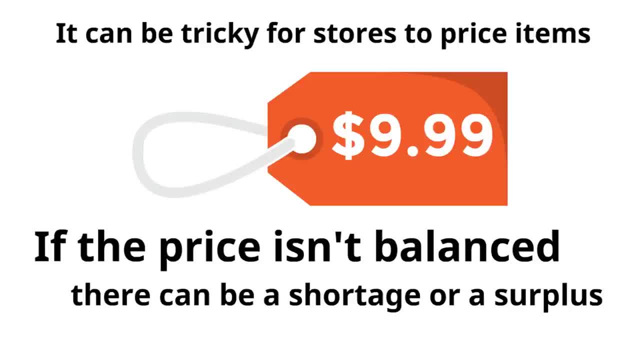 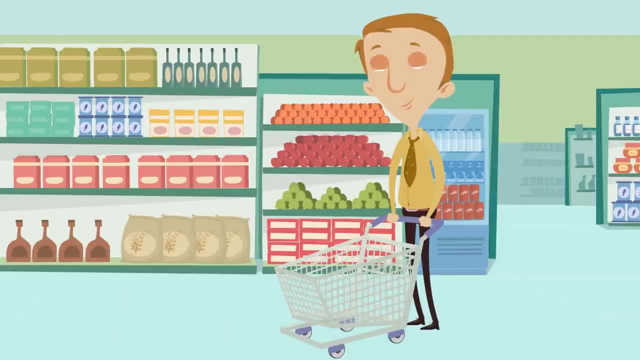 shortage or a surplus. well, I guess it's time to go back shopping. Wow, now you understand a shortage and surplus, and you understand a shortage and surplus, and you understand a shortage and surplus, and you understand that people who offer understand that. people who offer understand that people who offer goods and services have big choices when 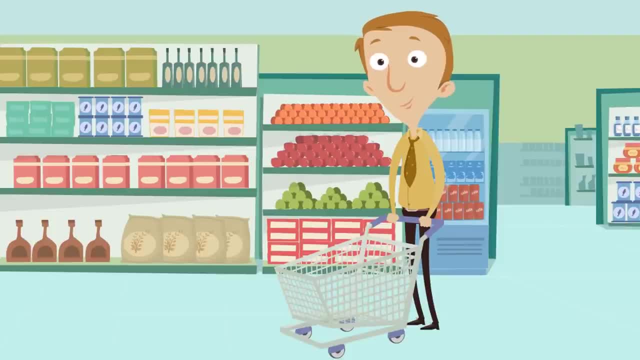 goods and services have big choices. when goods and services have big choices when they set the prices for things well. they set the prices for things well. they set the prices for things well. that's about it. so we'll see you like I. that's about it, so we'll see you, like I. 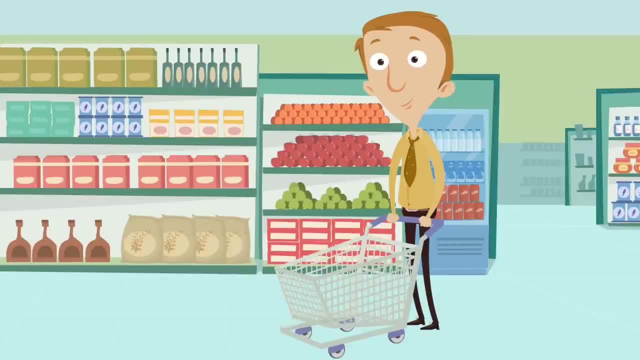 that's about it, so we'll see you. like I said I got it, I gotta go shopping. I said I got it, I gotta go shopping. I said I got it, I gotta go shopping. I don't know why you're still here, I got. don't know why you're still here, I got.